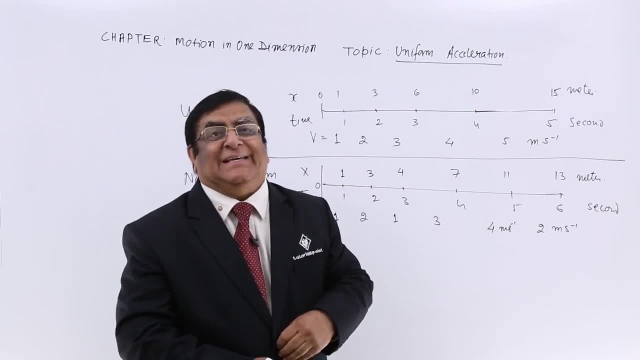 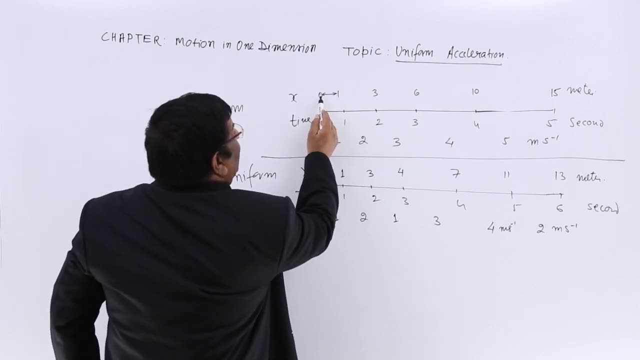 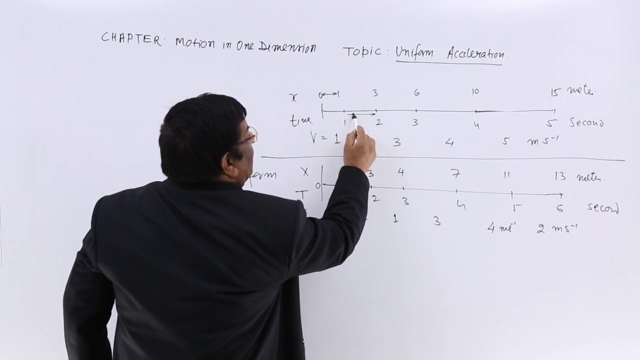 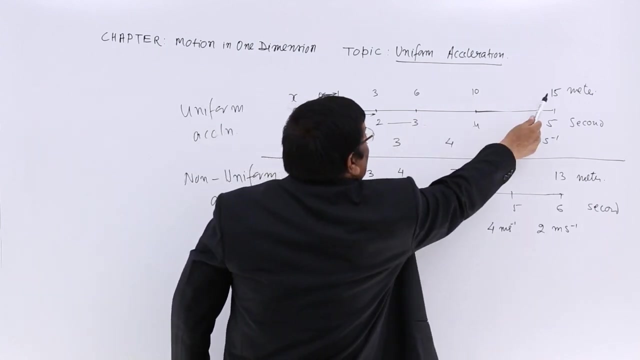 seconds. Then I have calculated velocity in each 1 second period. This 1 second period, the change in position is 1.. So 1 minus 0 divided by 1 gives the velocity. 3 minus 1 divided by 1 second, 6 minus 3 divided by 1 second, 10 minus 6 divided by 1 second. and. 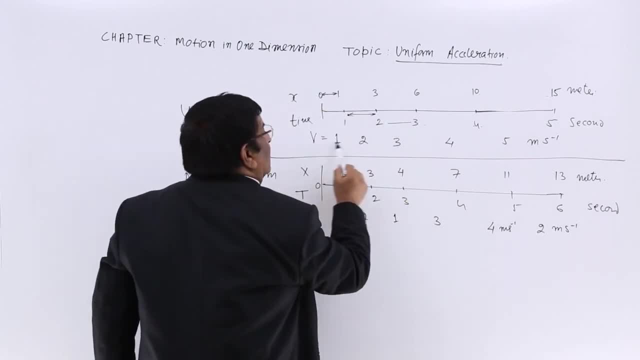 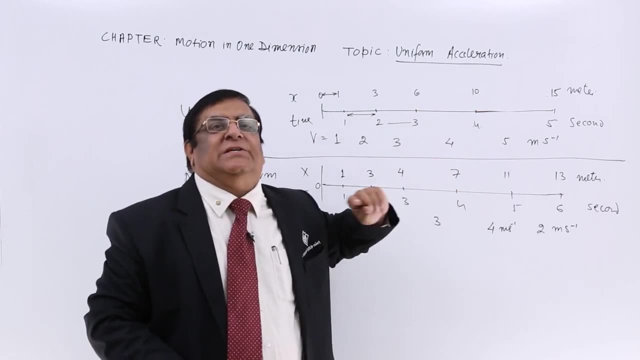 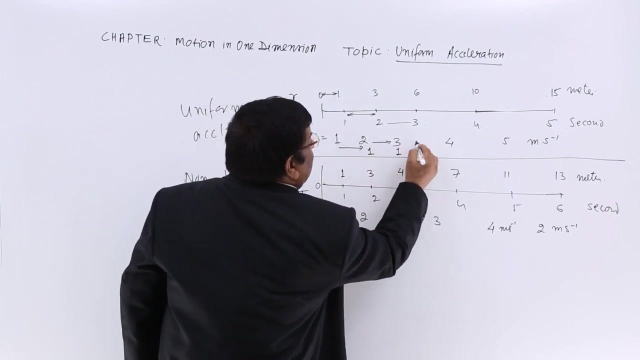 15 minus 10 divided by 1 second, That gives the velocity in each time period, average velocity in each time period. and now see the change in velocity: Here the change is 1, here the change is 1, here the change is 1 and here the change is: 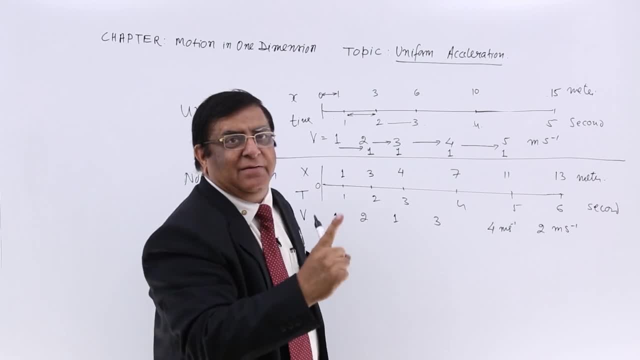 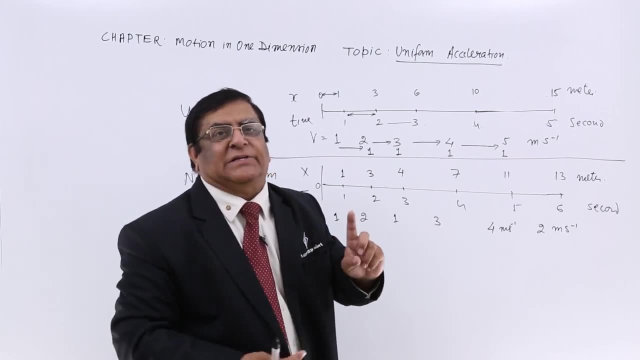 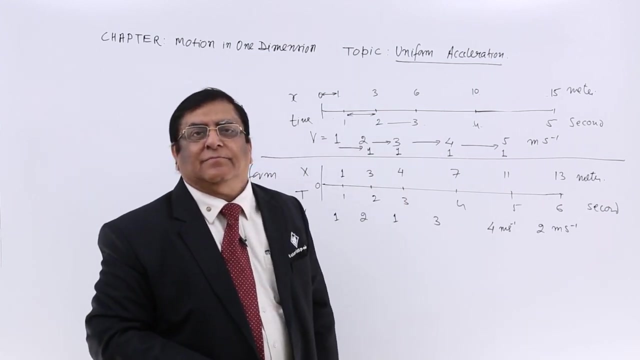 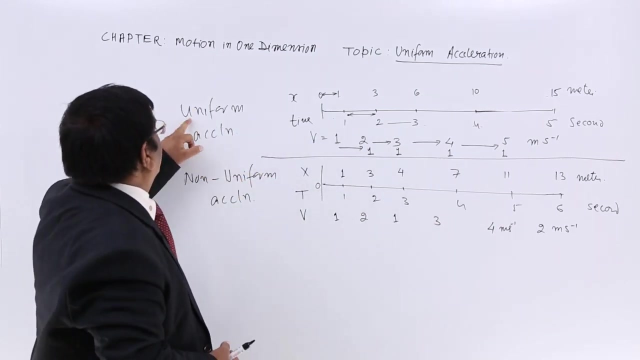 1. After every 1 second the velocity increase by 1, after every 1 second the velocity change by 1. We call it uniform change in velocity. For change in velocity we use the word acceleration. So this is uniform acceleration. Now see the second example: 1 second, 2 second, 3 second. 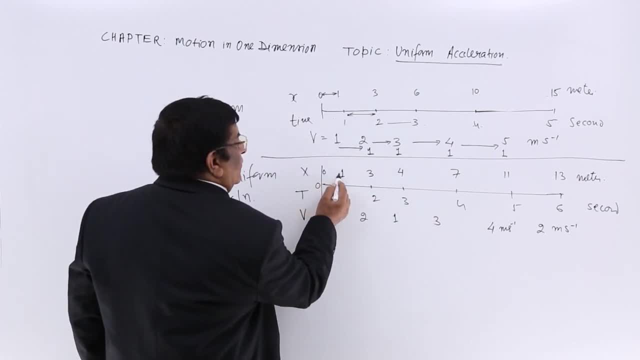 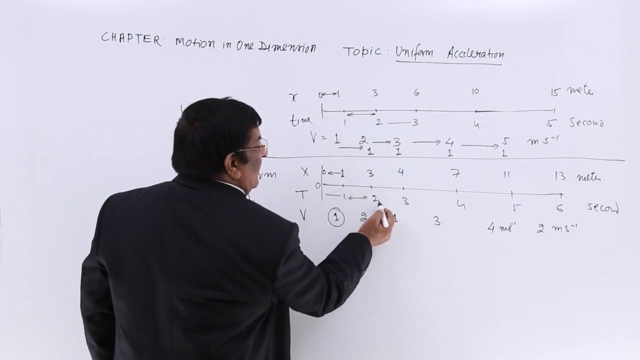 and this is the position Here. the velocity is 0 to 1,. 1 minus 0 divided by 1 is 1.. 3 minus 1 divided by 1 second is 1.. 2 to 1 second. 3 minus 1 divided by 1 is 2.. 4 minus 3 divided by 1 is 1.. 7 minus 4 divided. 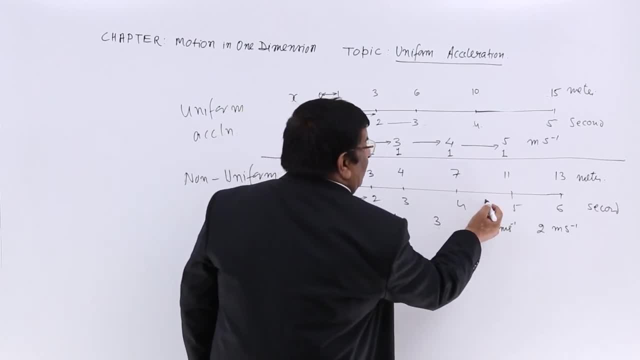 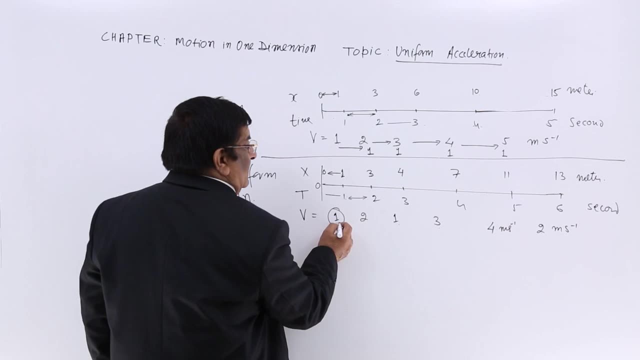 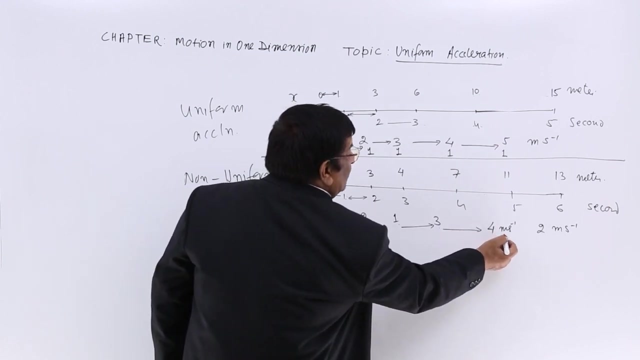 by 1 second, 3 and 11 minus 7. divided by 1 second, 4, 13 minus 11 divided by 1 is 2.. Here this is the velocity: 1, 2, 1, 3, 4.. Sometimes it is increasing and sometimes it is decreasing. 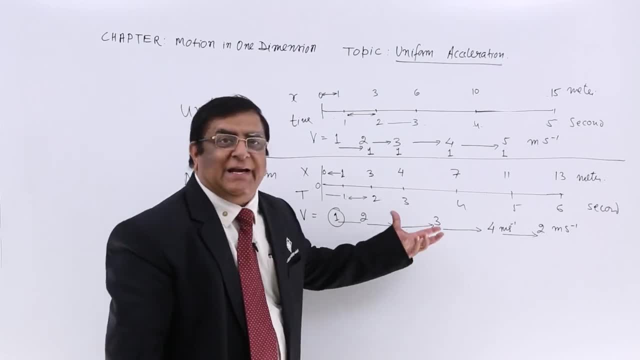 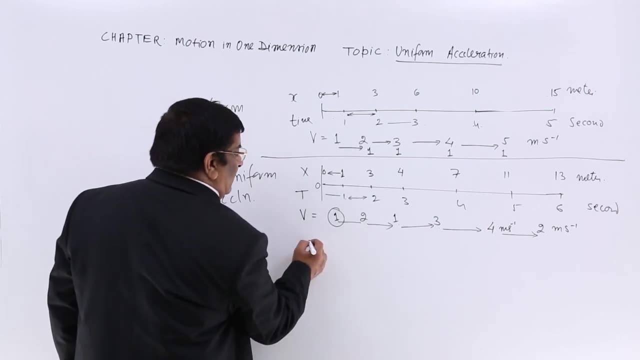 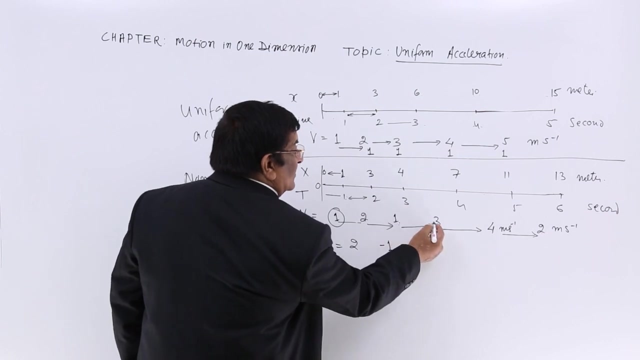 There is a variation, There is an acceleration. Always, Here is an acceleration. What is the acceleration? V2 minus V1. acceleration V2 minus V1 upon time, which is 1 second. So here acceleration is 2.. Here acceleration is 1 minus 2 minus 1.. Here acceleration is 3 minus. 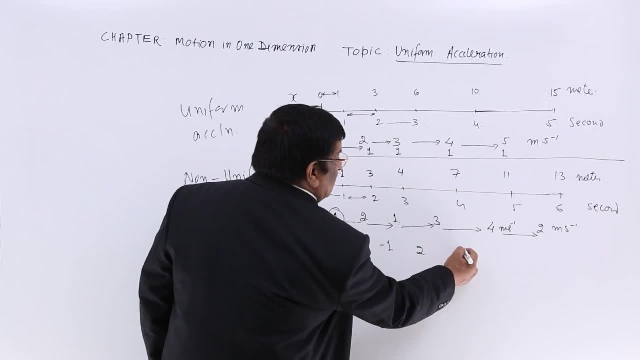 1., This is 2.. Here acceleration is 1., And here acceleration is 2.. So here acceleration is 1., So here acceleration is 2.. So here acceleration is 1., So here acceleration is 1., So here acceleration.